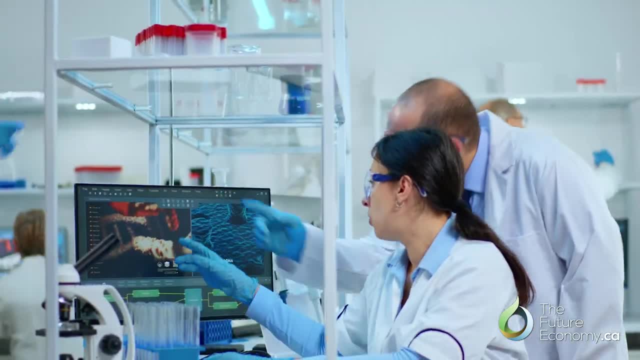 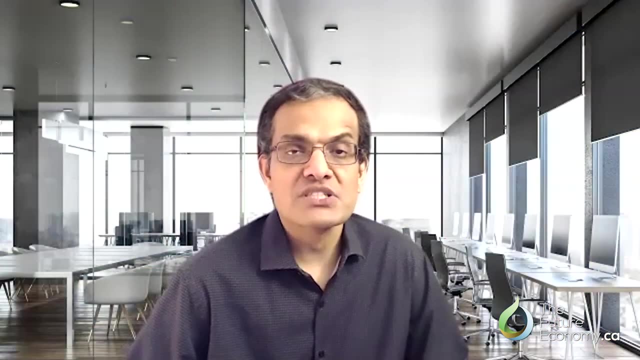 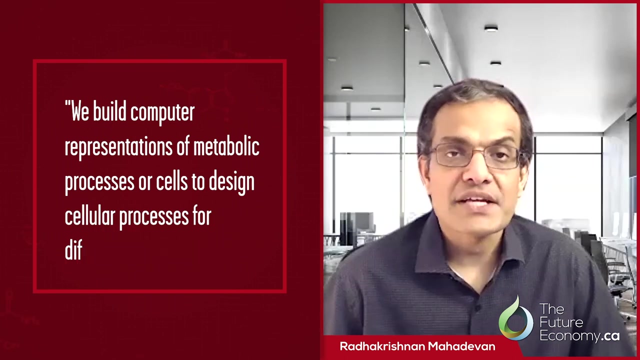 So what we do in our group is to make computer representations of these metabolic processes, or basically cells, and use these computer representations to actually design cellular processes for different applications. So one of the applications which we are working on in our lab as we speak now is the area of bionylon. 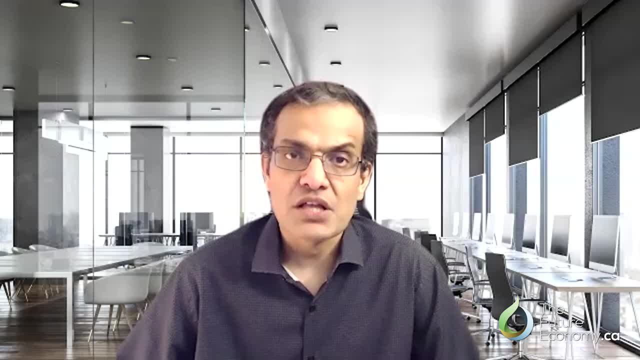 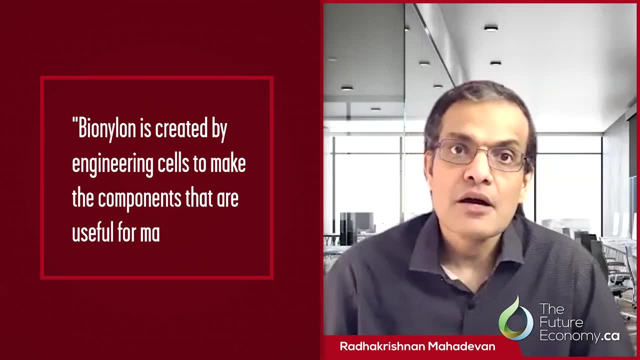 So in bionylon, what we try to do is to engineer cells to make the components that are useful to make nylon, And so nylon is essentially part of the clothes we wear. It's something that's you know, if you have a chair or something that you're sitting on, it's a part of the fabric. 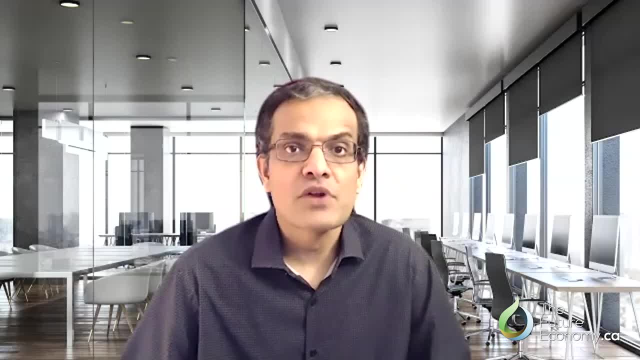 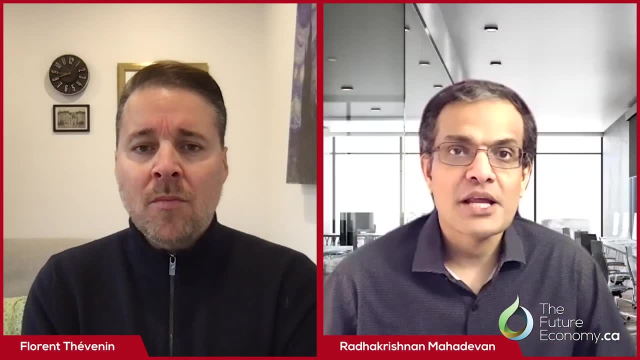 that's used to make these chairs, And so the idea for us is to take these pathways, put them into baker's yeast, so that you know, in theory, you can not only bake with the yeast, but you can also make the clothes that we wear with these yeasts, you know. 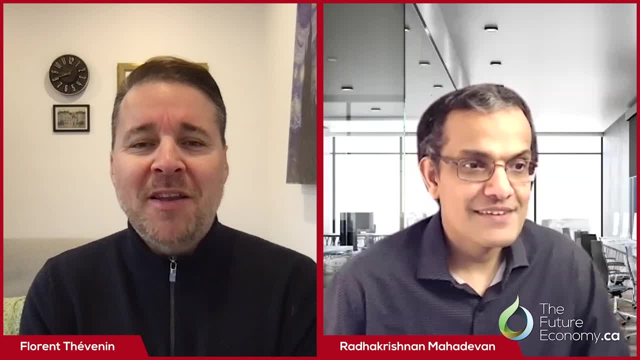 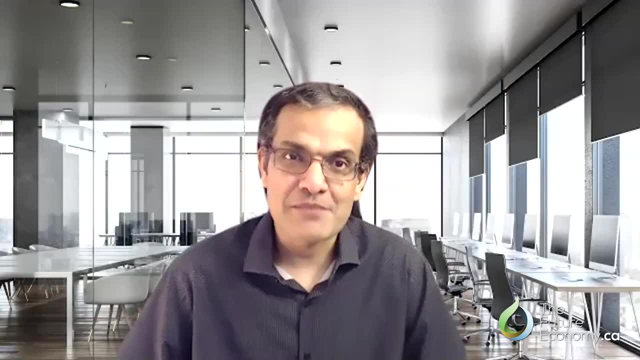 Fascinating, Fascinating. You put it very simply and of course it's much more complicated to make happen. right, Absolutely. There's a lot of processes that go behind actually being able to make yeast spit out nylon. First you have to actually understand what the pathways are and then you have to 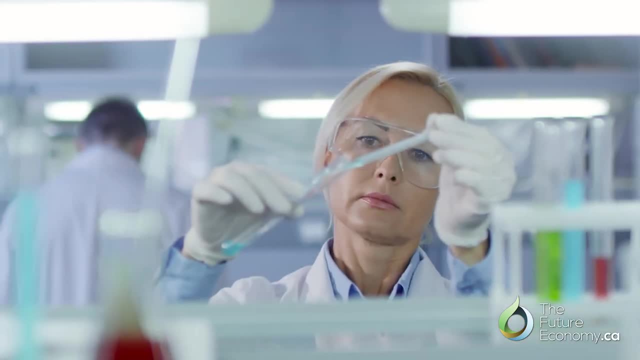 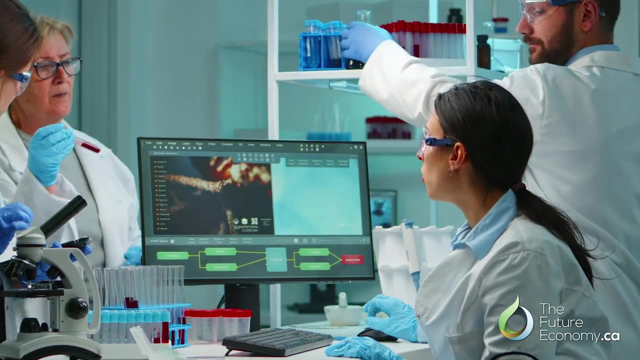 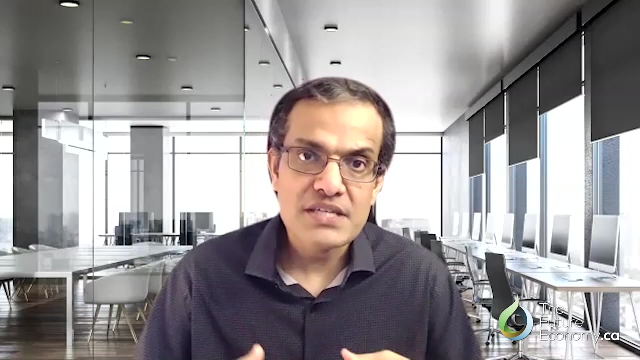 make sure that you can optimize them in some way, And so those optimization is something that we use. we do using model-based methods, Basically computer representations of these processes. Often what happens is that you know some part of biology sometimes is not very clear, right? So basically, there are multiple mechanisms. 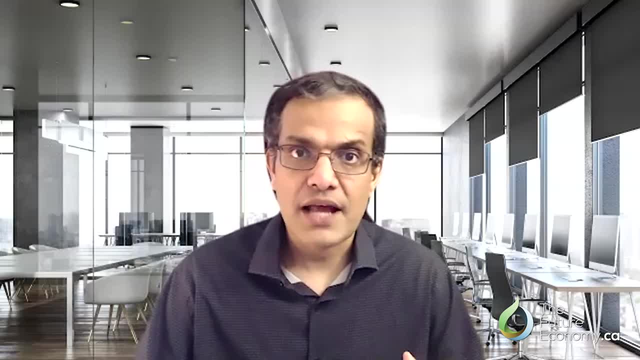 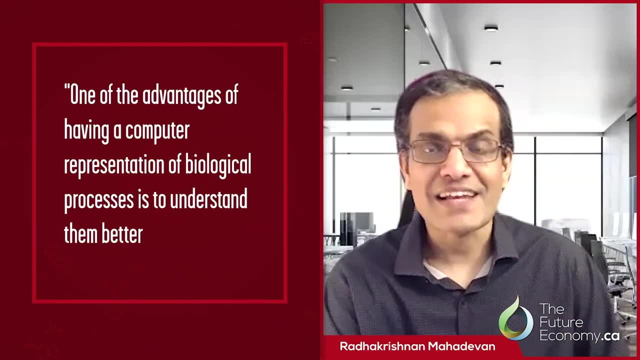 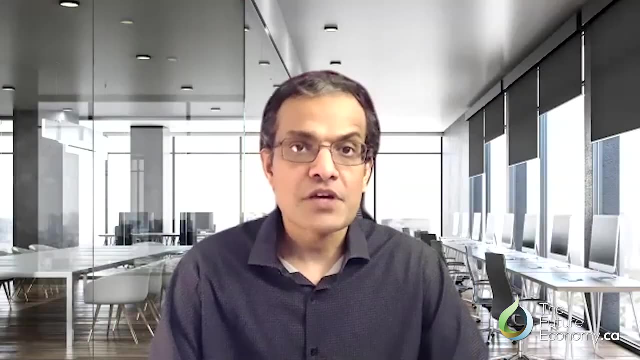 by which biology can the processes in biology can happen, And one of the advantages of having a computer representation for that is to understand things that are not really well understood. So basically, if there are multiple hypotheses underlying a biological event, we can use a. 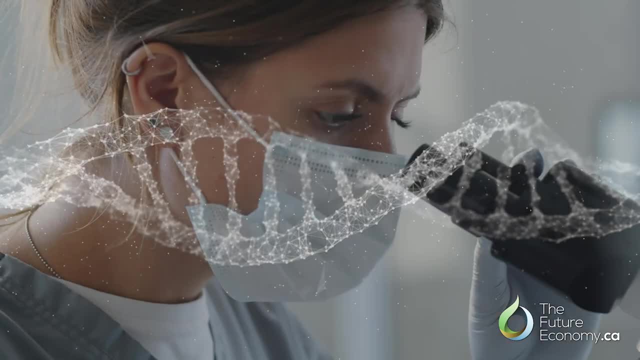 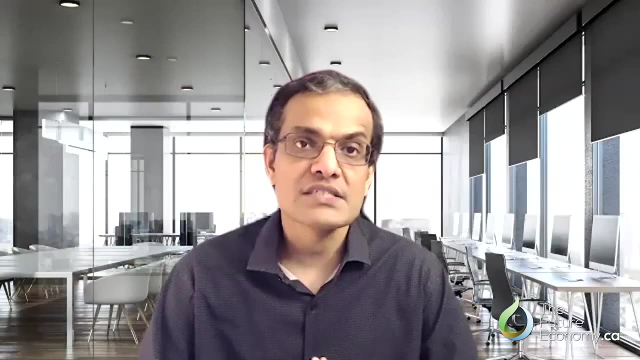 model-based framework to actually test them, And so that's what we're doing, And so that's one type of implementation that can do that. So it's not gonna be a long and long process, but you can test them out and then try to figure out that one hypothesis is actually true, and that can 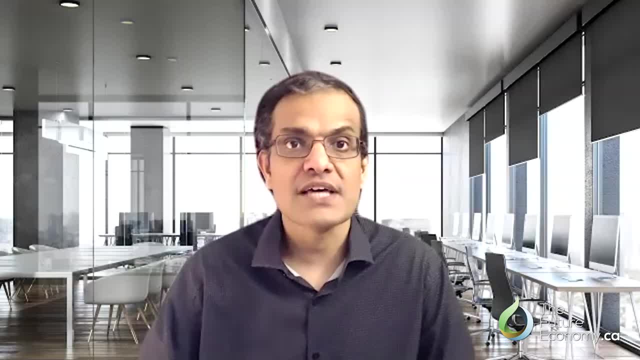 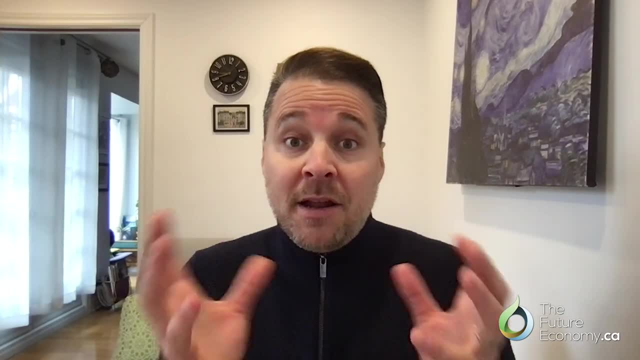 actually provide more fundamental knowledge and, of course, improve our understanding of biology, which can eventually lead to improved computer representations, and, of course, improve designs and applications, And I guess that's an area where things like artificial intelligence or machine learning, where Canada is quite strong, help right. 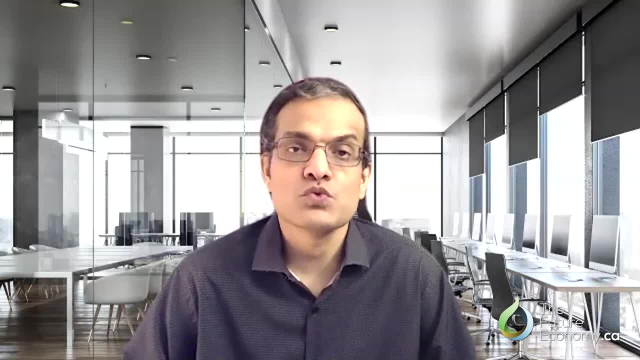 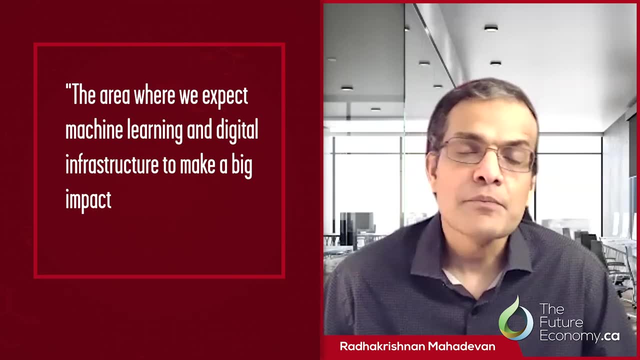 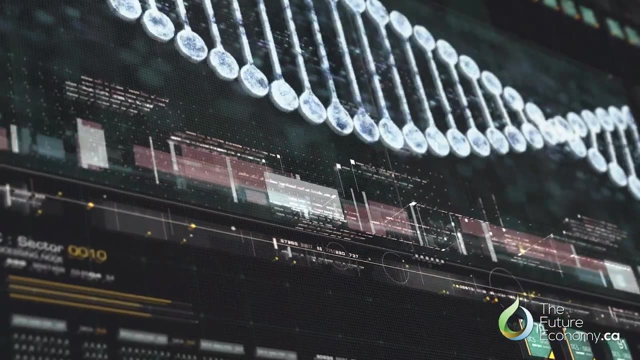 Absolutely So. the the the area where digital infrastructure to make a big impact is in the design, modeling, optimization and design of cellular processes. So, basically, people are able to design, using these AI and machine learning tools: better strains, better proteins, better enzymes, better catalysts that can actually 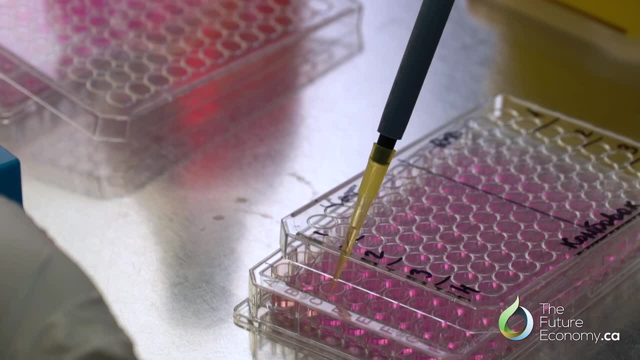 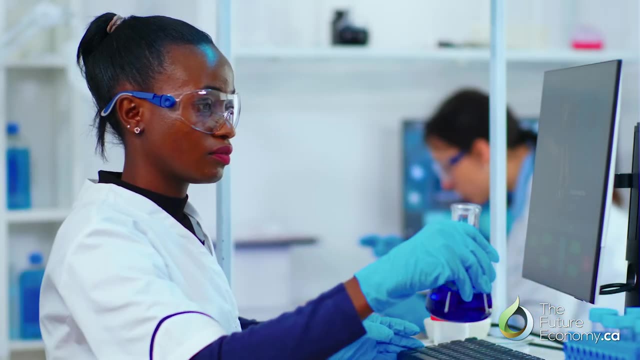 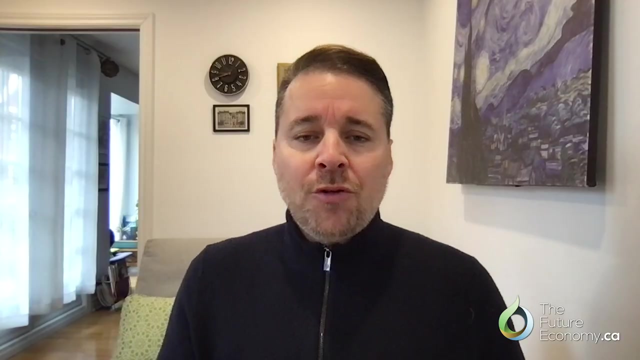 catalyze the processes that are required to make these products And, in general, the combination of AI and machine learning, along with the advances in biology side with respect to us being able to rapidly make new genetic designs, Sort of like the speed at which the latest vaccine for COVID were developed, I suppose. 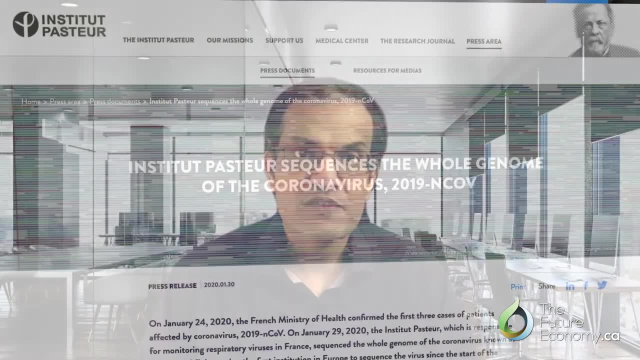 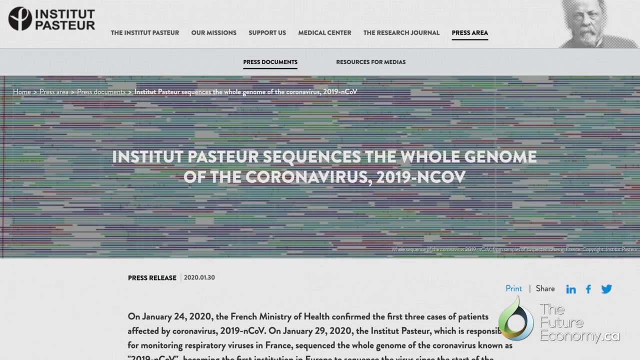 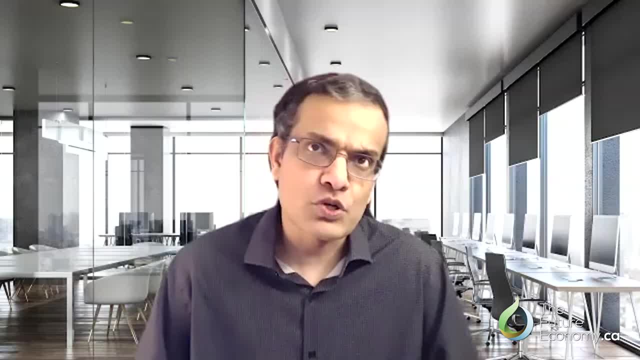 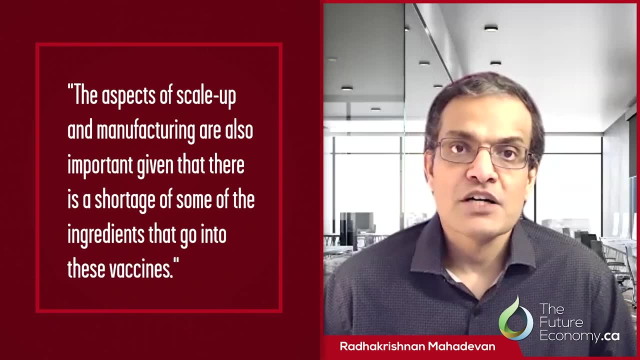 made And then the rest of the processes and the regularization of the vaccine. the mRNA design was the delay as opposed to the design side. Of course, there is the aspect of scale-up and manufacturing, which is also important, given that there is a shortage of some of the ingredients that 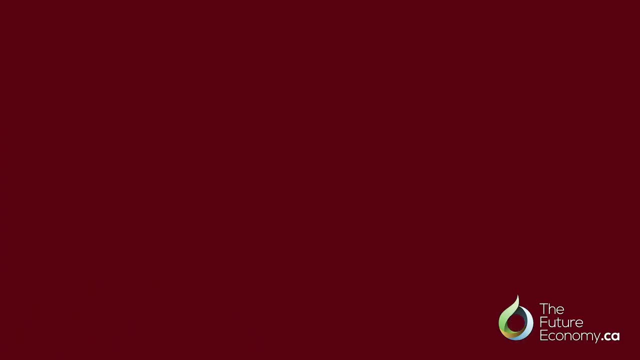 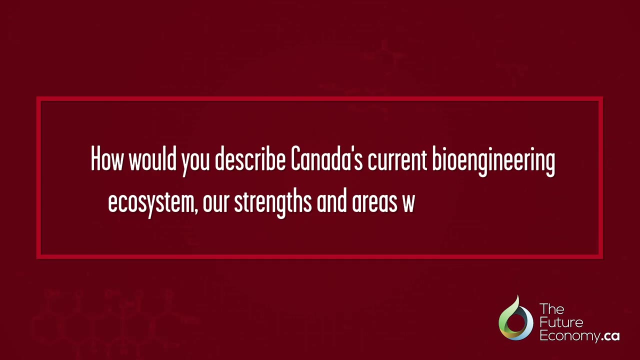 go into these vaccines. So how would you describe Canada's current bioengineering ecosystem? What would you say are some of our strengths and what are areas of improvement in that area? Yeah, so that's a great question. I think Canada is actually, in my opinion, very well positioned. 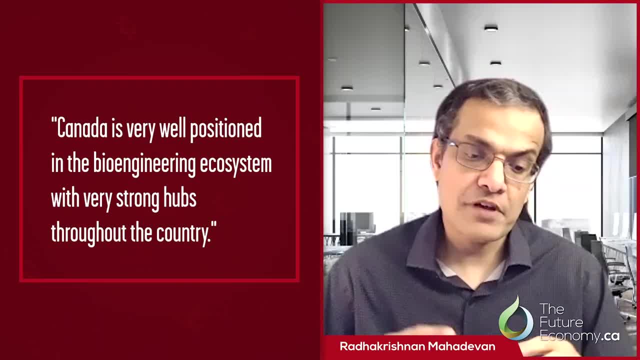 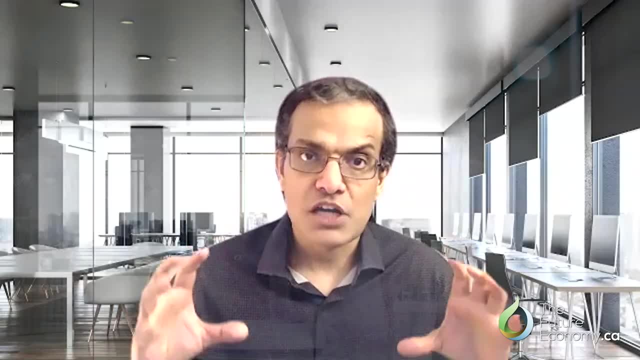 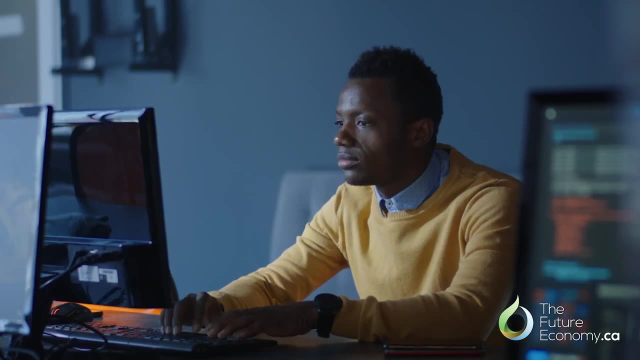 in the bioengineering ecosystem. There are, I feel like, very strong hubs in certain locations. So, for example, in Montreal, Toronto, Vancouver, there is a cluster of companies, there's a cluster of research groups that are actually doing work in this area And, separately from that, Canada. 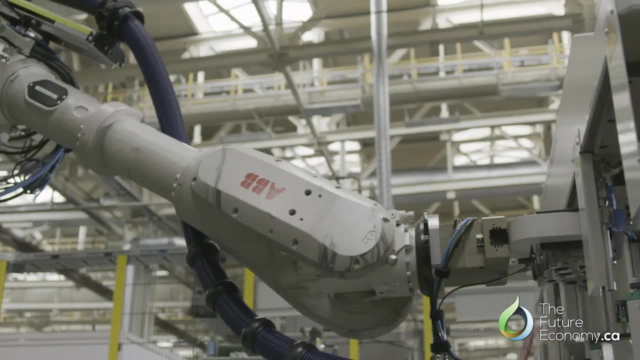 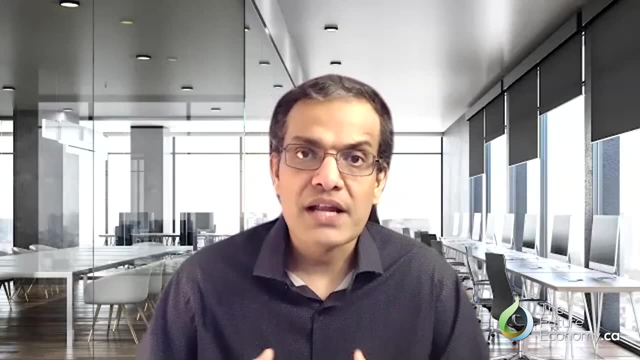 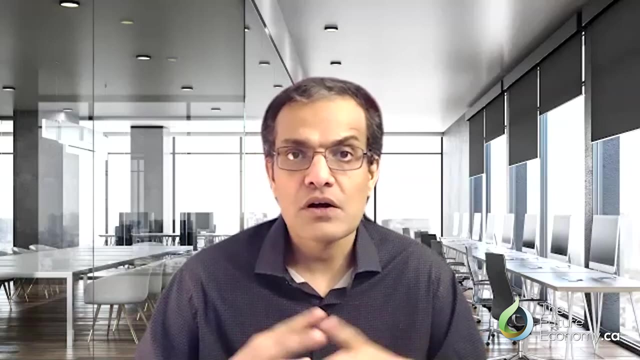 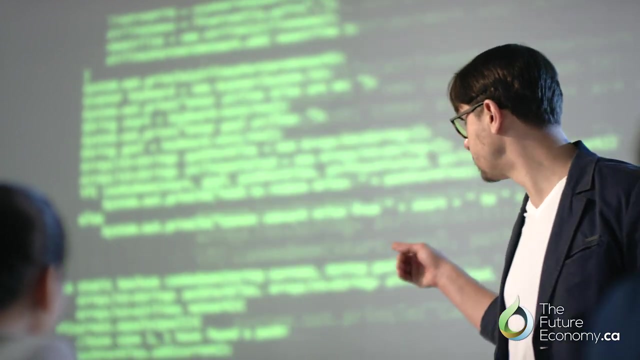 also has historic strengths in automation and machine learning, in robotics etc. So that's led to high-throughput data and basically methods to interpret and learn these high-throughput datasets. So Canada has really strong points in all of these components: in the genomics area, in the machine learning area, as well as in the high-throughput data. 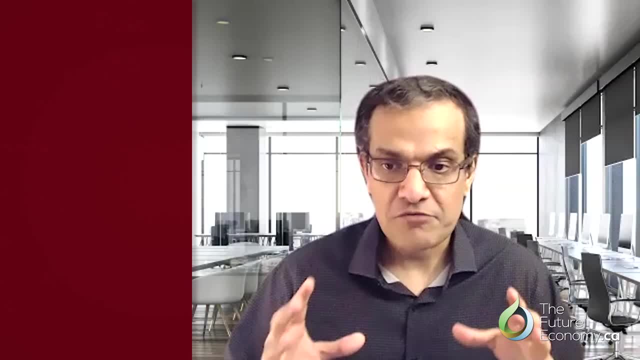 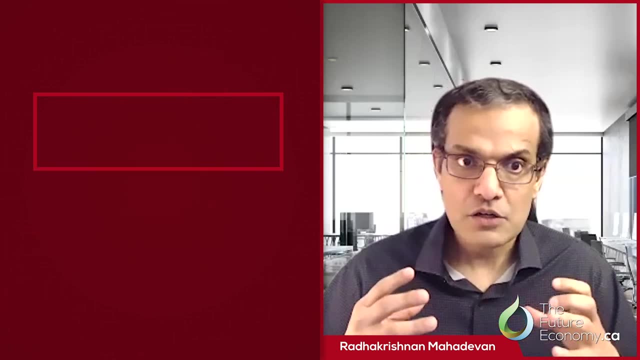 slash robotics, slash omics area. You know, in Canada there's also some weaknesses, right? I think the weakness is primarily, I would say, on the infrastructure side, right, I mean, there are certain groups like the NRC where there is centralized places where they could. 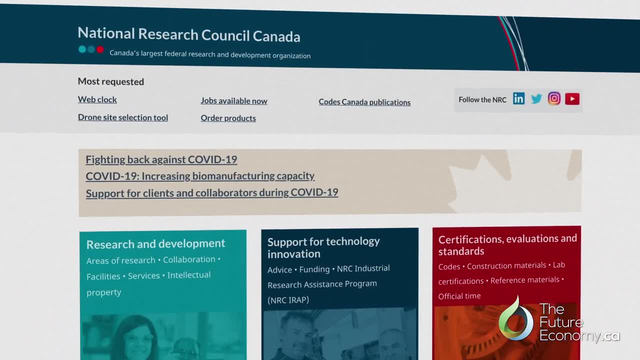 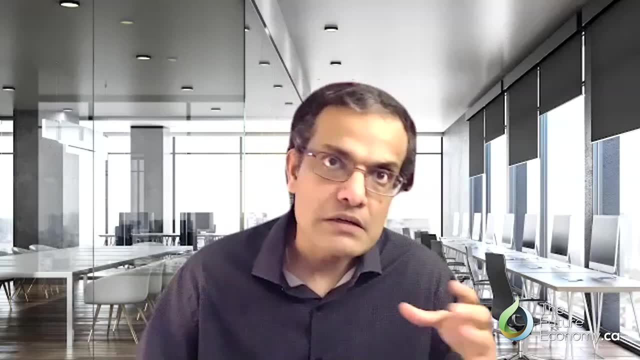 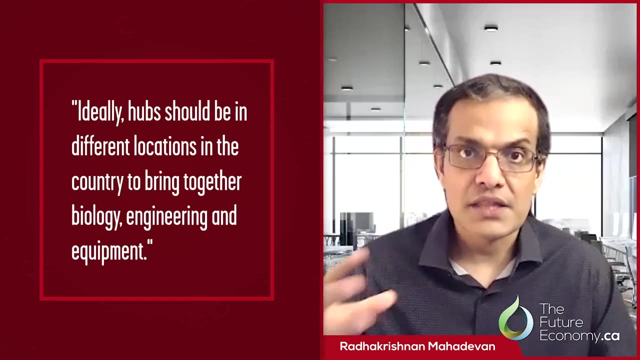 scale up manufacturing etc. But I think, like such hubs are not more broad spread in the Canadian context, So ideally you know you'd like to have hubs in different locations in the country that actually bring together the biology and the engineering and the equipment. 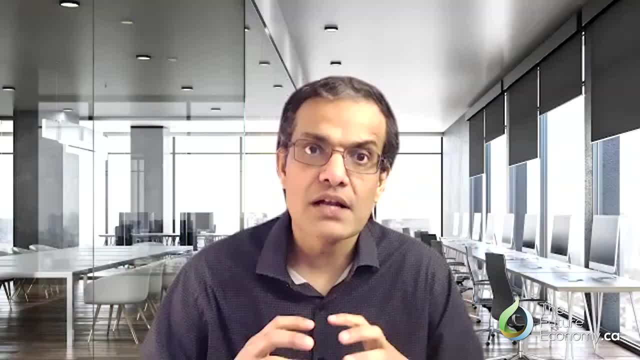 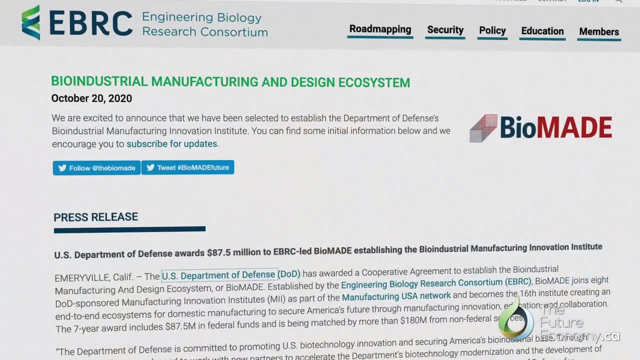 and space together right, And so there is fewer examples of that here, whereas you know in the US and other places you know, there is a lot more investment. For example, in the US, we recognize that this is a need And I know that hundreds of millions of dollars have been. 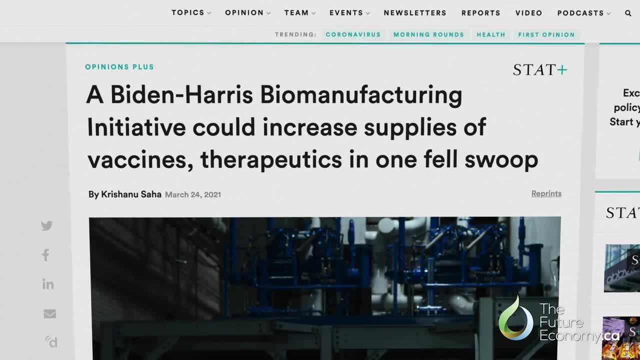 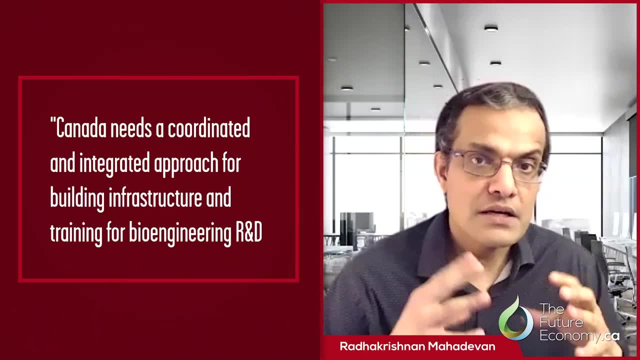 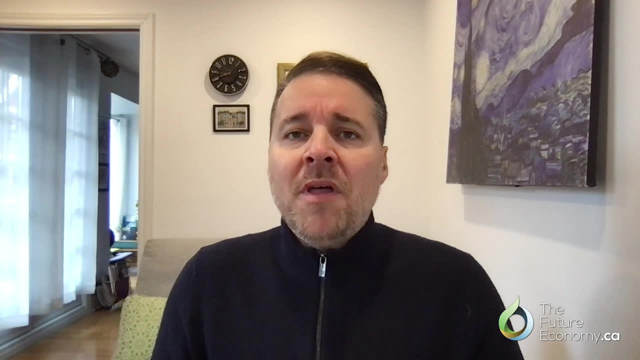 spent in terms of setting up a national biomanufacturing ecosystem right, And so I feel like this is something that Canada needs: a coordinated and an integrated approach for doing infrastructure, for doing training and translation for bioengineering R&D. So, with that in mind, and the fact that, as you pointed out earlier, we have strengths in many 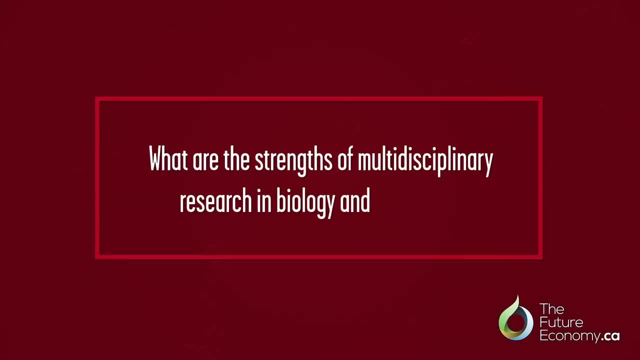 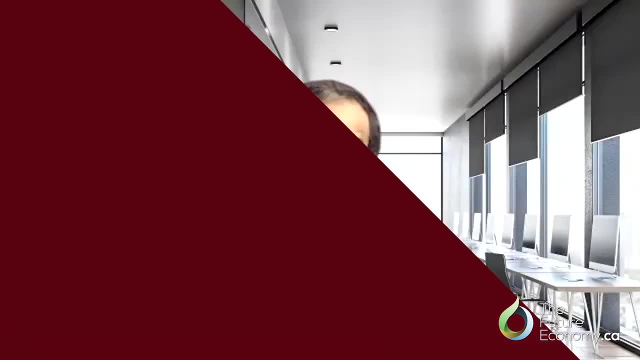 areas, for instance, artificial intelligence. Can you speak to the benefits of that, The benefits of multidisciplinary research, particularly as it applies to biology and genomics? Absolutely, So. that's a really, really important topic. So what's happened in the last? 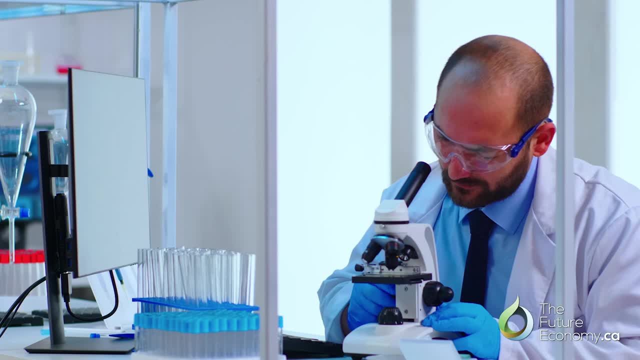 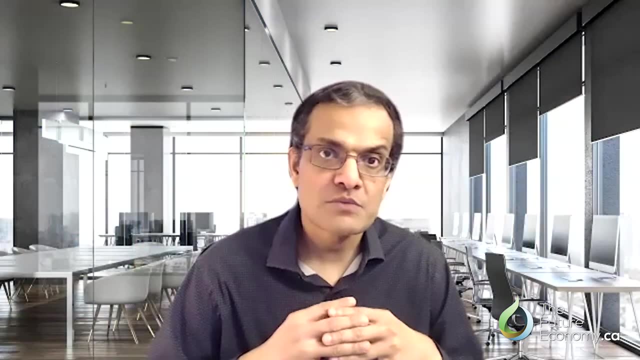 few years is that biology has become seriously information rich. right, So you'll be able to, like you know, do an analysis at what we call the genome scale. And so genome is basically at the level of genes, And usually many organisms have thousands of genes, So every gene, every. 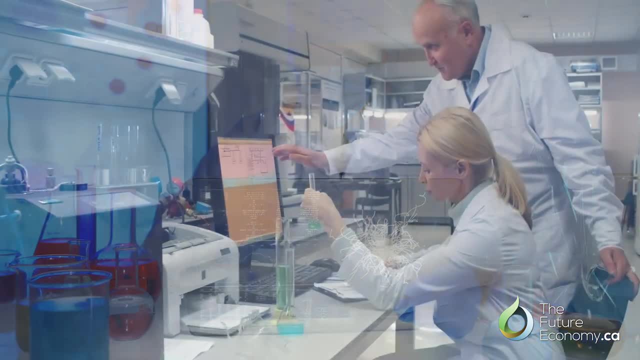 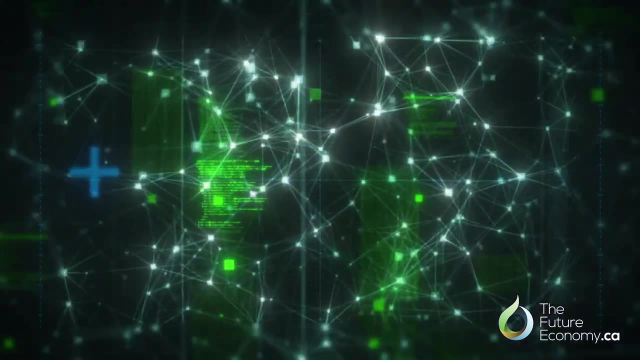 organism. we have thousands of data points, And so we have a lot of data points, And so such data, especially if it's generated in a high-throughput manner, right lends itself to like machine learning and data-based methods, And so there is a combination of biology. 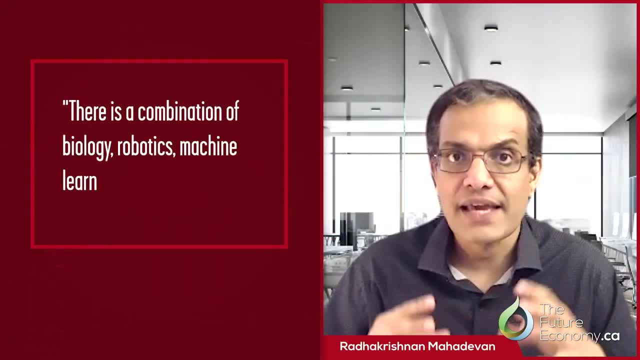 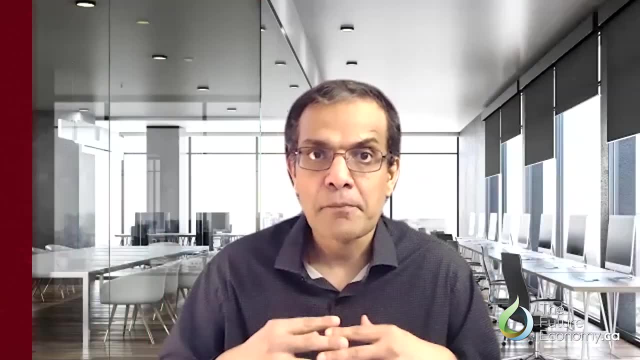 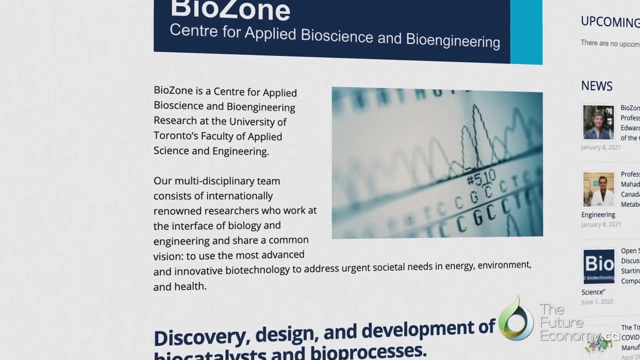 robotics and machine learning slash AI. that is required to advance bioengineering in the future. So it's definitely really multidisciplinary And I should point out that you know at the center that I am a part of, which is BioZone, is actually a multidisciplinary. 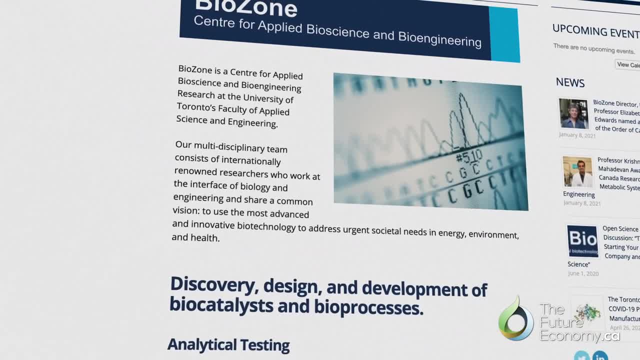 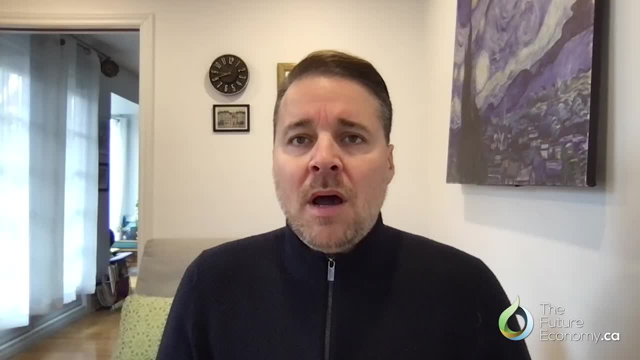 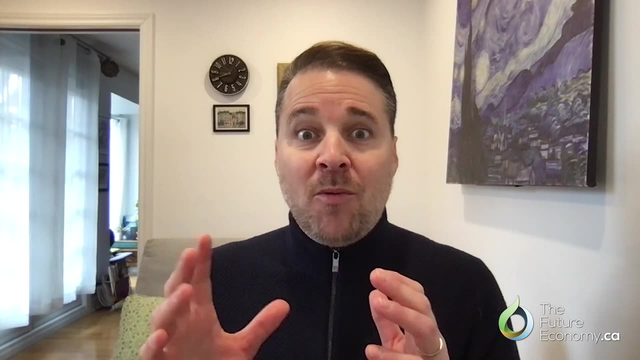 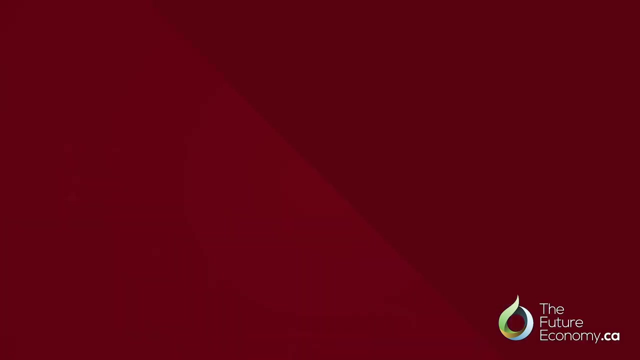 center where faculty members from different areas come together and tackle some really important problems in sustainability. Now we're obviously in the middle of a global pandemic, and there have been previous ones, And we pretty much know for sure that there will be more, and some even say perhaps even more often. Why is genomics important in 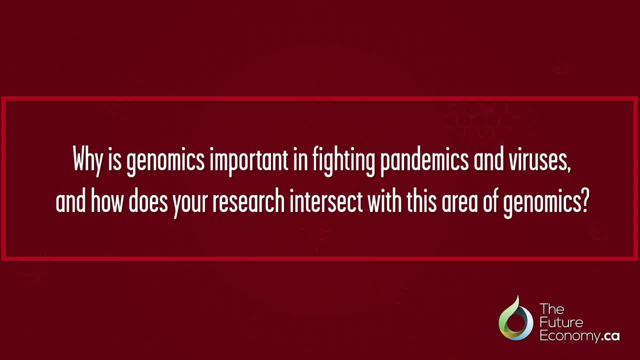 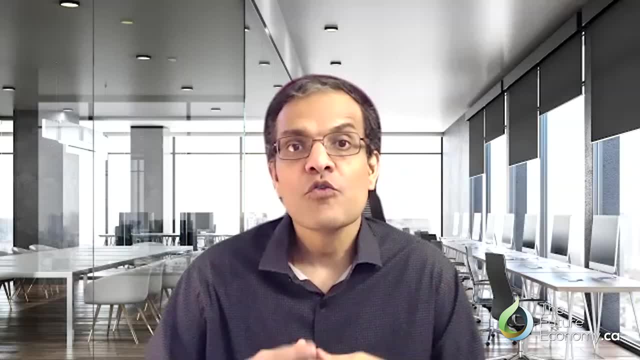 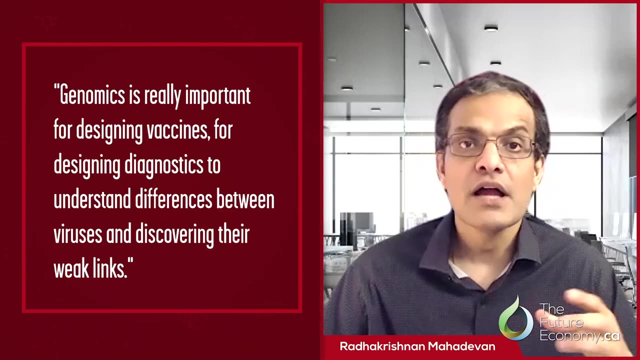 fighting pandemics and fighting viruses, And how does your research, your research, intersect with that field of genomics? Why is the genome sequence important? Because it's really important for designing vaccines, and for designing diagnostics too, to understand how this is different from existing viruses. 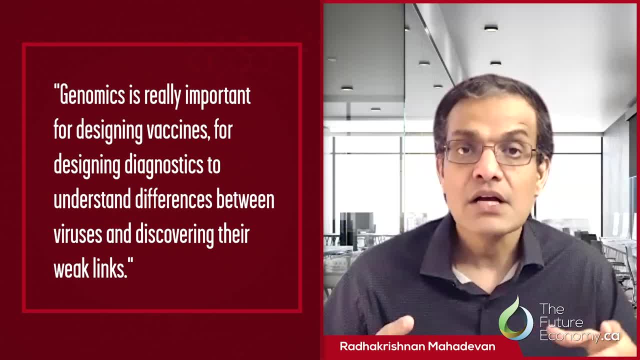 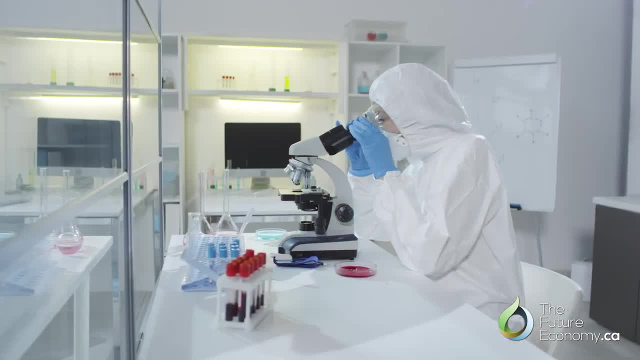 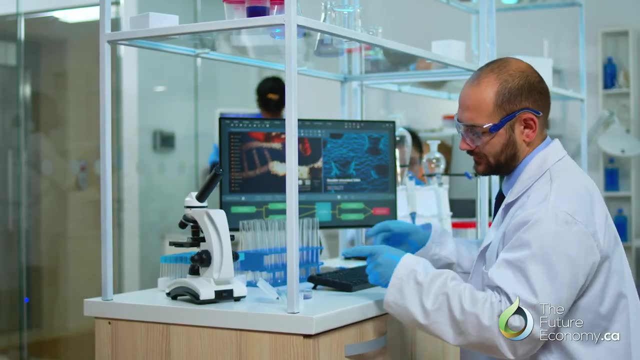 and what are the weak links associated with this virus? So in that case, right, you really need to actually have the genomic information so that you can understand whether a particular virus is spreading and whether a variant of the virus is spreading. And if there are mutations in the virus, are there ways in which these mutations can allow? 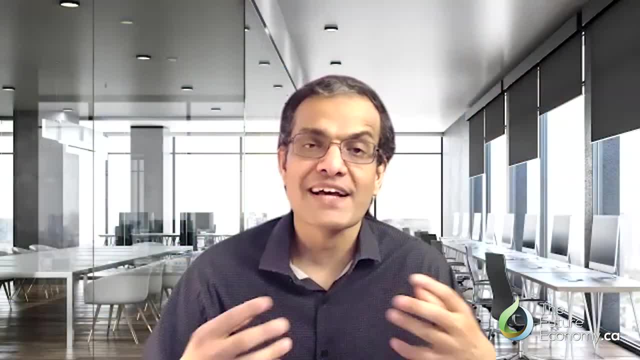 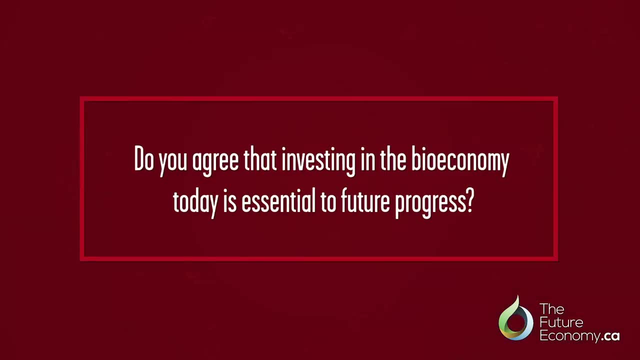 the virus to escape the antibody treatment or the vaccine treatment. During our interview with Dr Lakshmi Krishna this morning, she mentioned that it was very important today to invest massively in the bioeconomy for future progress. Do you agree with that? 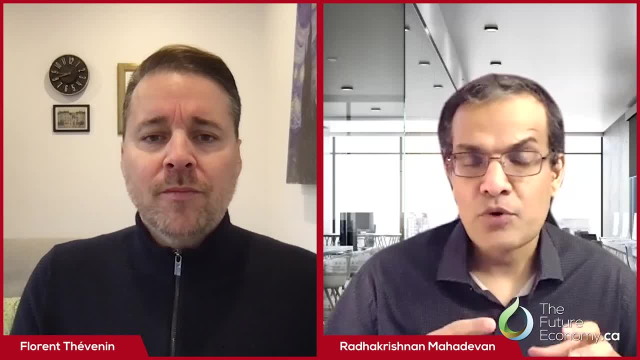 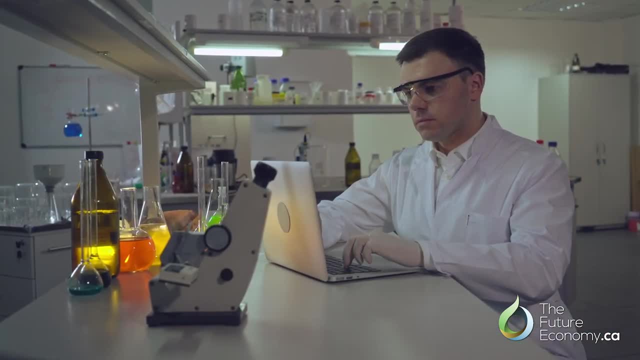 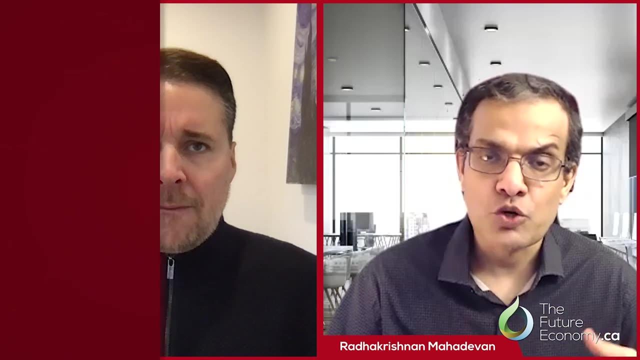 Yeah, absolutely. So. I would say that this is the time to actually invest in biomanufacturing and bioengineering research, primarily for two reasons. One is that there has been a lot of developments that has given us unprecedented access to what's going on inside the cell in terms of genomics, in terms of us being able to 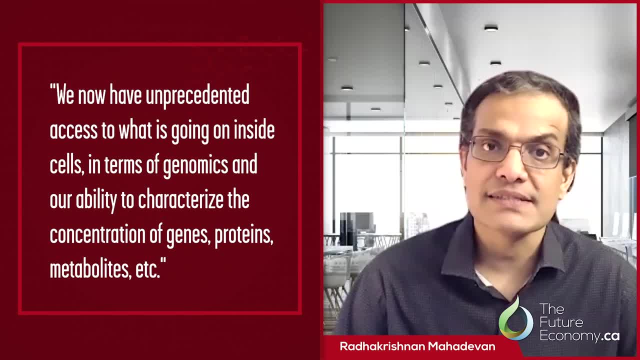 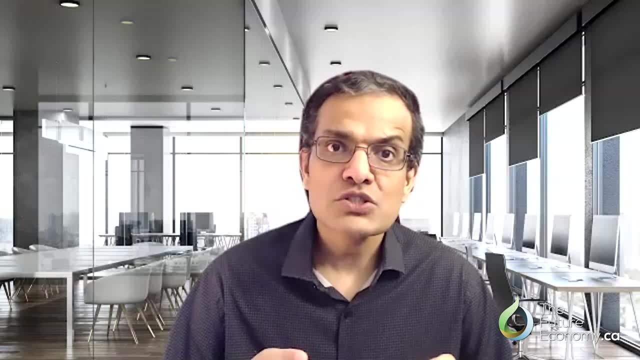 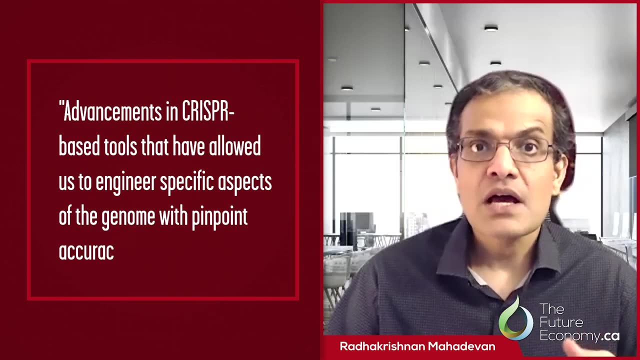 characterize the concentration of genes, proteins, metabolites into the cell. Separately. there has been advances in the area of CRISPR-based tools. that has allowed us to engineer with pinpoint accuracy specific aspects of the genome. So these two events have created an opportunity for us to 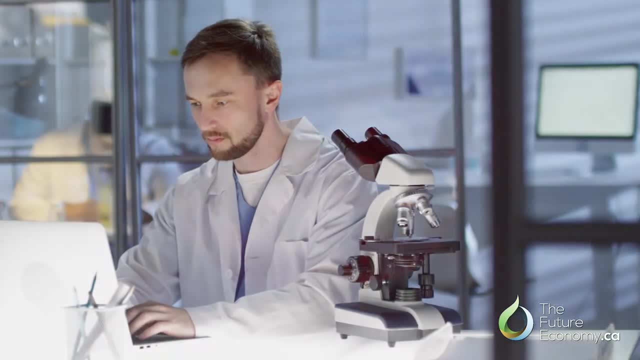 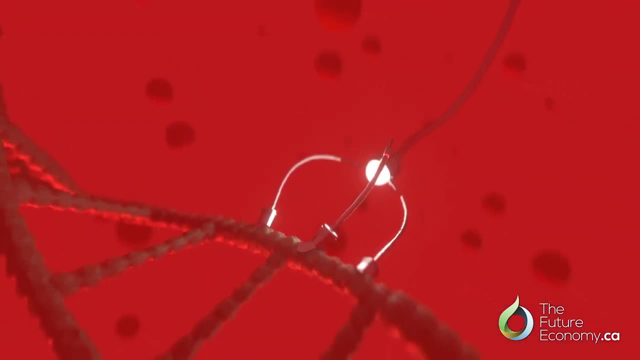 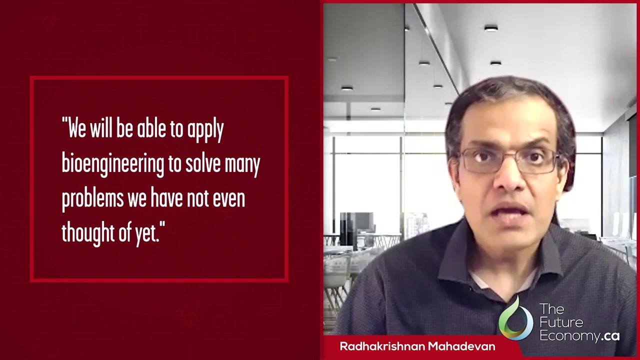 engineer these microbes or communities or human cells at an unprecedented, if you will, a level of ability and in a very targeted fashion, And that will allow us to apply bioengineering for many, many problems that we are not even thinking of, And some of them people are talking about. 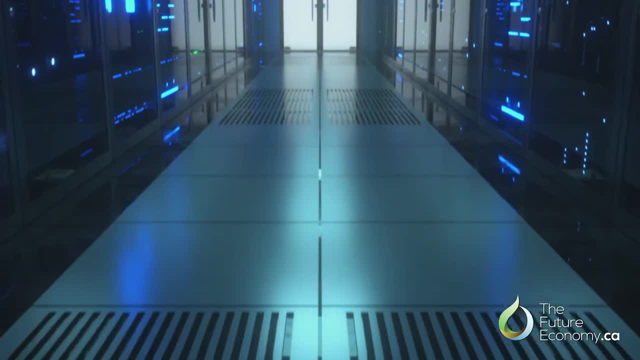 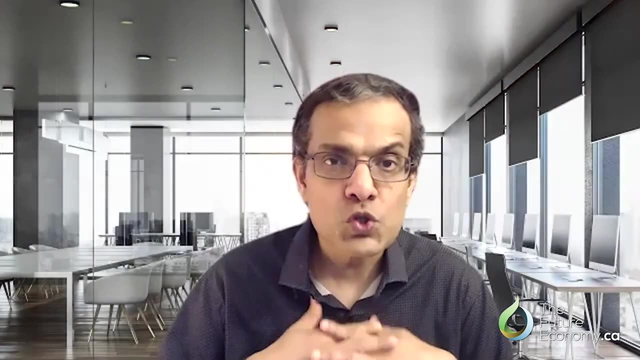 information storage. So instead of storing in books and whatnot in a library, people are talking about storing such information in a genome and locking it away. So there is a whole slew of applications that we have not even thought about. that will become possible with the. 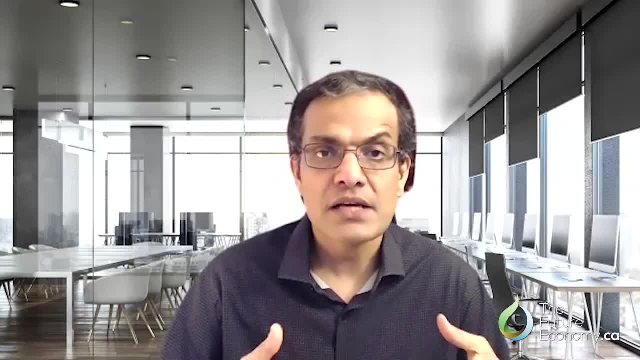 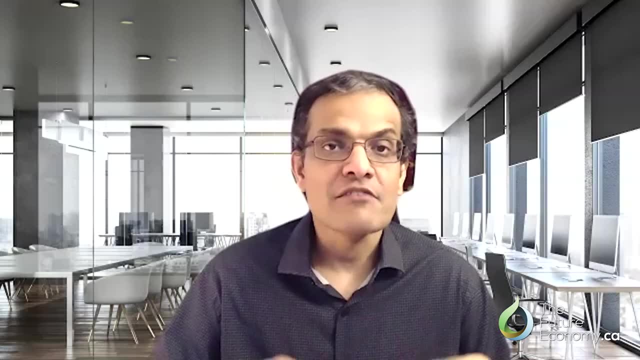 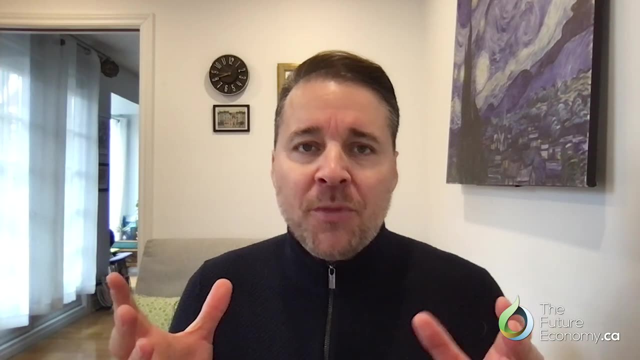 advances in bioengineering and basically CRISPR-based tools, And we hope that Canada is able to take advantage by investing in this particular area at this particular time. If you had 30 seconds to pitch someone or even a group in a position of power, 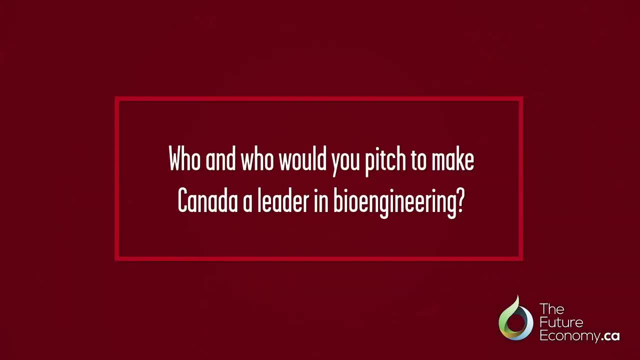 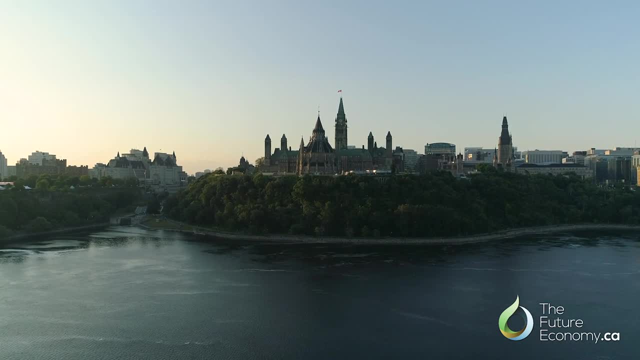 to make Canada a leader in bioengineering. who would you choose to pitch and what would you urge him, her or them to do in 30 seconds? Yeah, absolutely, I'd love to have 30 seconds with the Prime Minister or the Minister of Science and Innovation, if you will, And I would. 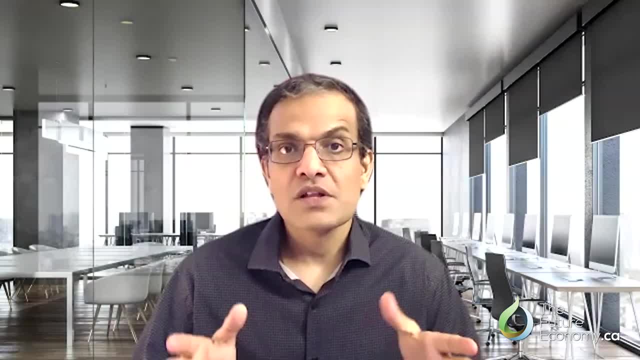 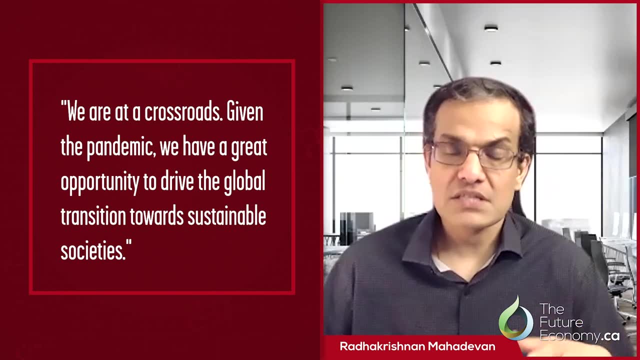 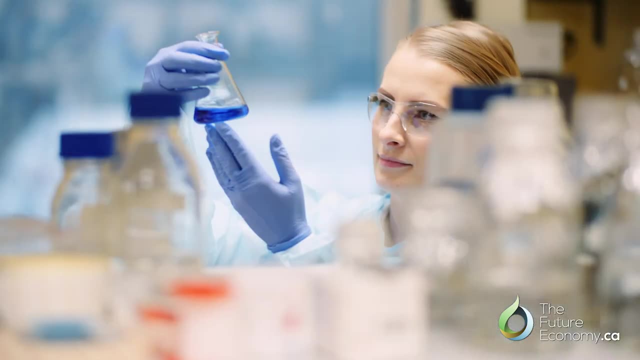 say to them: look, we are at crossroads here. Given the pandemic, we have a great opportunity to drive this global transition to sustainable societies, And so that's a push that's coming. And Canada, if you will, has the strengths in genomics. It has the 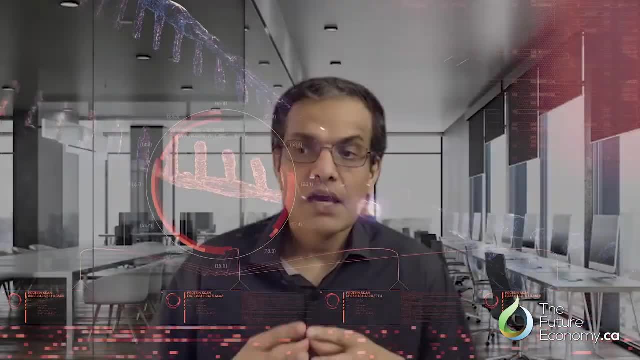 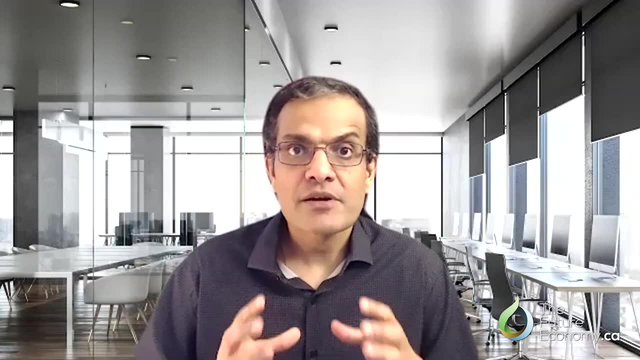 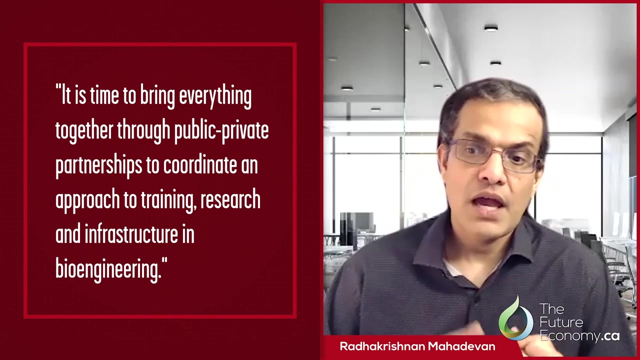 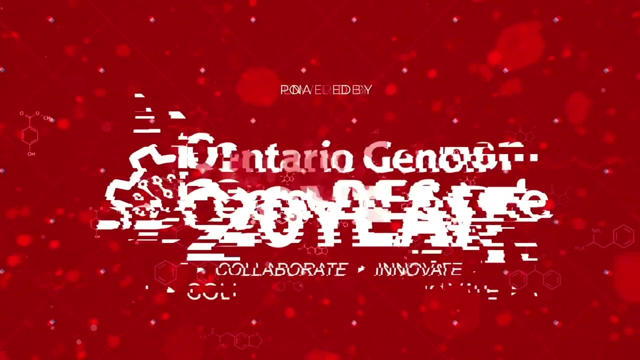 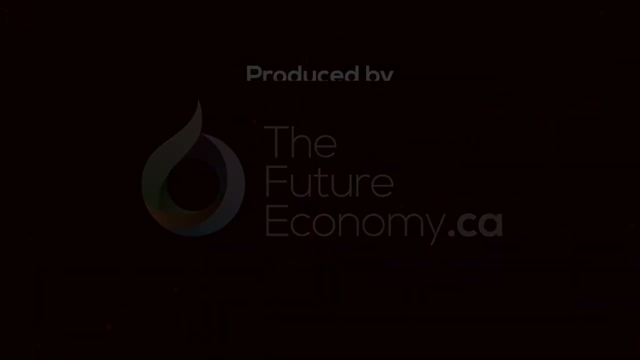 strengths in artificial intelligence and machine learning, etc. And it's time to kind of bring everything together and put together public-private partnerships that can get a coordinated approach to training, research and infrastructure in this area. Thank you so much for joining us.